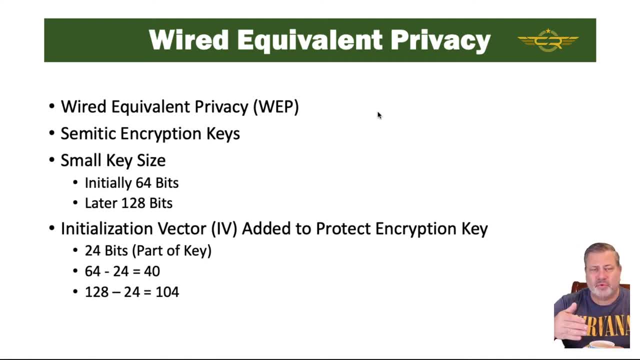 128 bits, which was still way too small to make this thing secure as it was designed, and we'll see that. So it had a thing called an initialization vector that was added to protect the encryption key, and that was 24 bits and the IV was actually part of the key size. So if you had initially 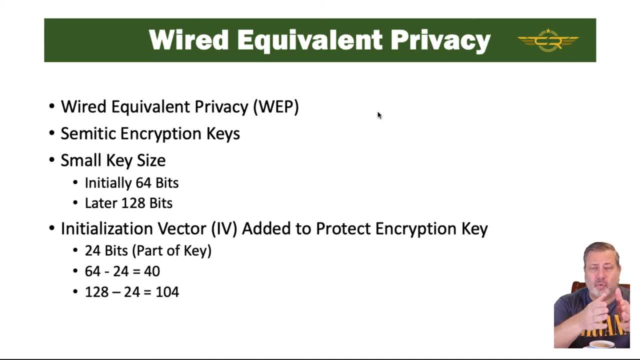 like in 1999, we had a 64-bit requirement- Couldn't be longer than that, and part of that was this IV or this initialization vector. That means your key size. your encryption key size could only be 40 bits, and even when we increase that to 128 bits, that meant your key size could. 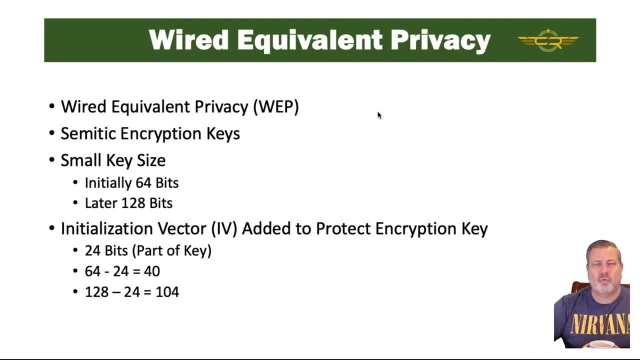 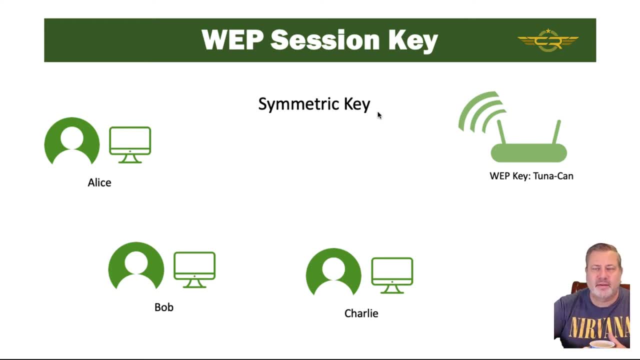 be 104 bits and we'll see. even with that, it wasn't quite strong enough the way this thing was designed right. So again, symmetric key. when we looked at the session key that everyone used to connect to the network, it was a symmetric key, which means that if we look at our 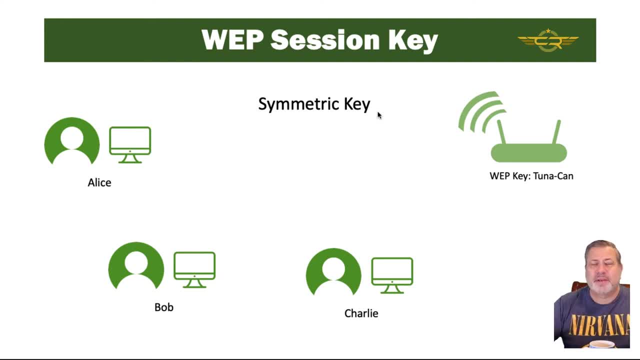 access point up there. its name you know. its web key is Tunican. That means when Alice connected she had to use a web key of Tunican. Bob used the web key of Tunican and Charlie used the web key of. 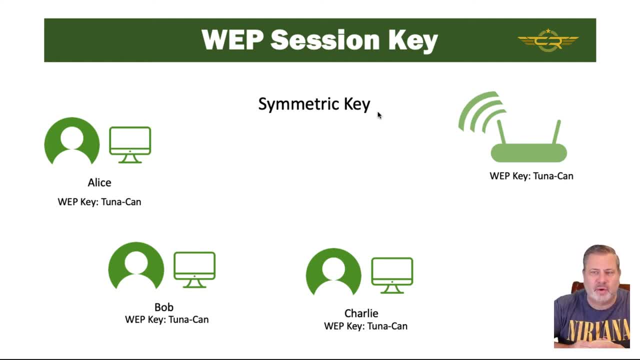 Tunican, Everybody used that same web key and I know that's a crazy web key, but just wanted to make the point. Everyone uses it. So if you had a hundred users and one of them left, you would have to change that session key on everyone's computer and on the access point. So obviously that made 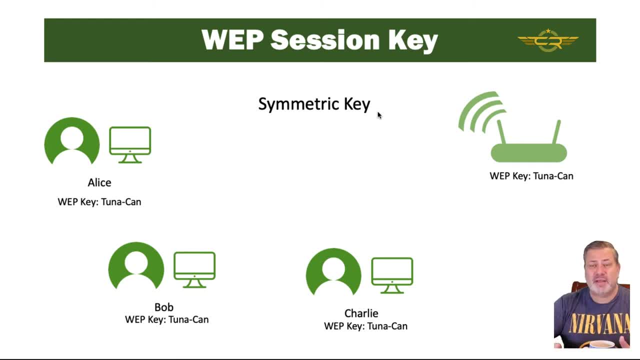 it a problem, and the fact that everyone used the same key meant that it was a little bit more vulnerable as that key transitioned the network because everyone used the same one. So let's look at a little bit how this process works when we're using this IV, what the IV actually does for us. 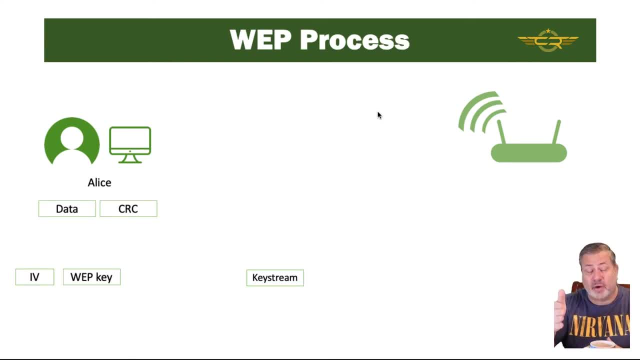 right, We're gonna say Alice is gonna send some traffic across the network, right? So she starts out and she's got a data packet, which is shown at the top there, and a CRC or a cyclic redundancy check, and that just makes sure that the data is correct. right, So it's a mathematical. 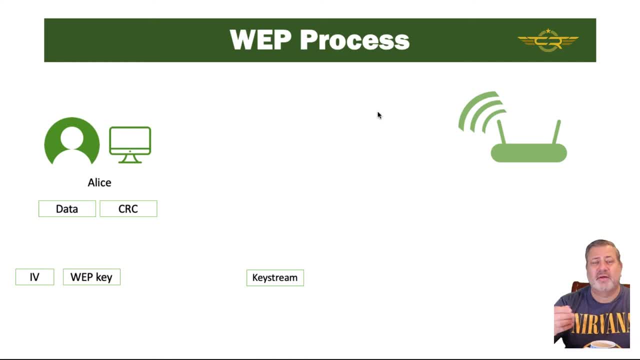 function on the data, to give it a value, so that we can check on the other end to make sure that the data is correct. That's packaged together, That's made into one group, the data and the CRC, and then on the other side, on the wireless protocol side, on the kind of the web side. 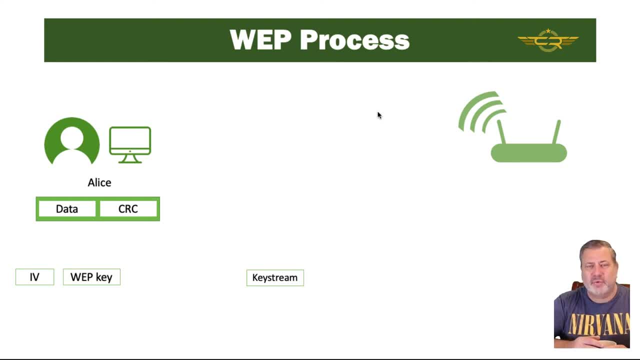 we have our web key, which we know in this case is Tunican, and then we have an initialization and that's gonna provide some what they call equivalent to salting right. So it's gonna add some value to the key so it doesn't look the same every time that it goes across the network. So the 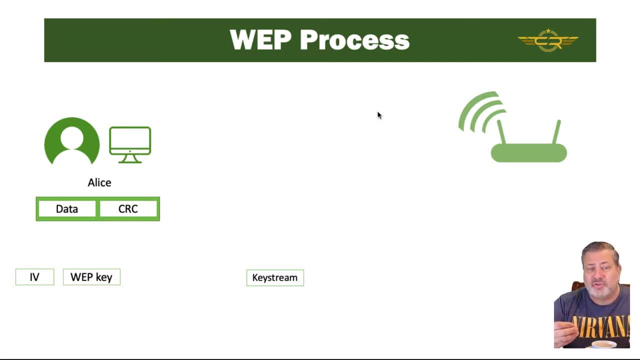 IV and the web key are kind of put together and they're kind of munged and there's- it's not very a technical term, but the IV allows the web key to be changed a bit or salted, So those kind of. 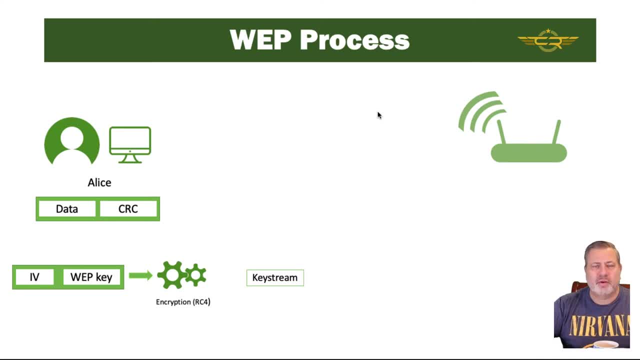 are put together and then they're run through the actual encryption system and then they're encrypted and then it establishes that path. And so you know, we're forever going to fries, p kind of futses, and we try to charge. you know a little. 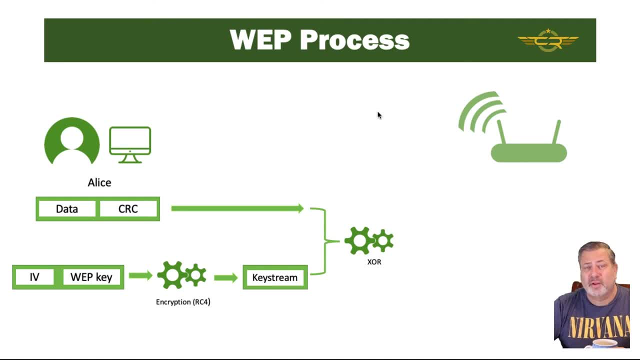 bit of signal to it across the wireless network. So we have ciphertext getting ready to go across the wireless network and now one of the big problems with this is that we had to also send the initialization vector with the ciphertext, because that's going to be a value that changes and at the receiving end they're going to need that. 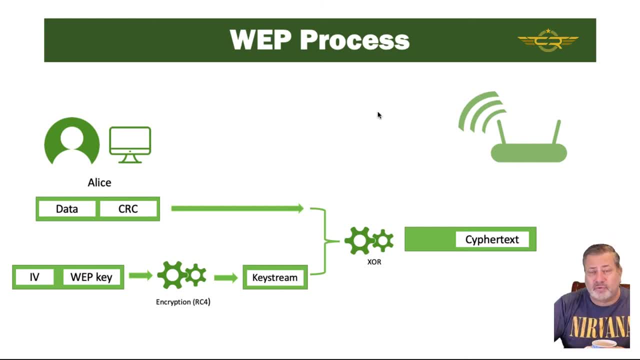 to be able to decrypt or go back through this process backwards. So we have to append the IV in plain text to the ciphertext that's going across the network. So that's one of our first problems. Now we've got the initialization vector in plain text, with our ciphertext going across the network and there it. 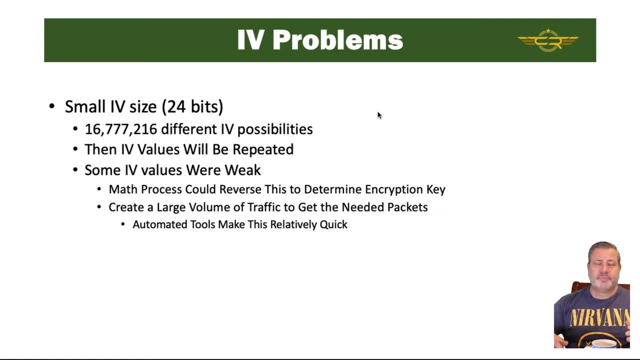 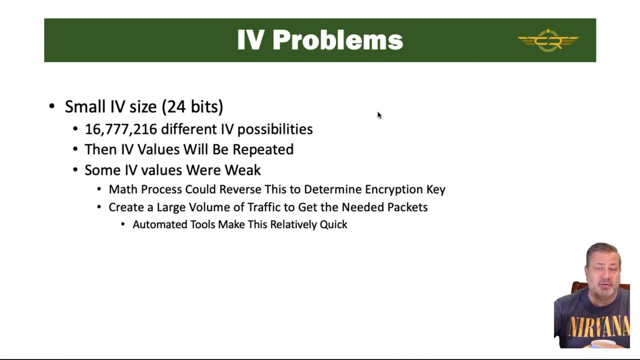 777,000, 777,000, 777,000, 777,000, 777,100, 777.. If we go through that number, then of course that will be the largest number that will ever happen before an IV is repeated. Some of these IV values are actually weaker than other. 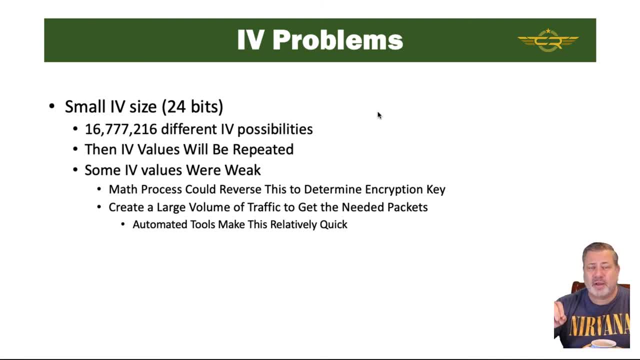 IV values and we can use a math process to reverse this and determine the encryption key. So all we need is to push a large volume of data across the wireless network and then we can figure out these IVs and we can figure out the encryption key. 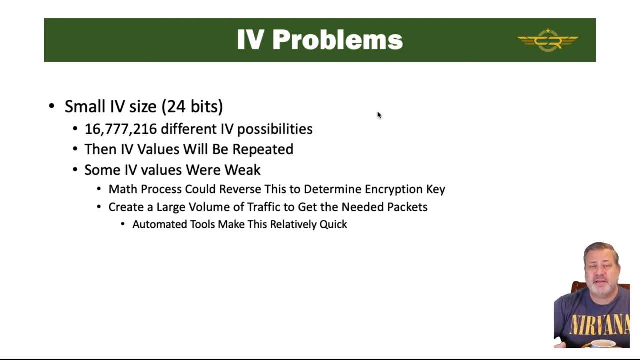 So when you are doing that on the use case, Especially if we can get IV values to repeat, and if they're the weak IV values, then we'll more easily be able to break the encryption key, break the web key and figure out what the actual encryption key is. 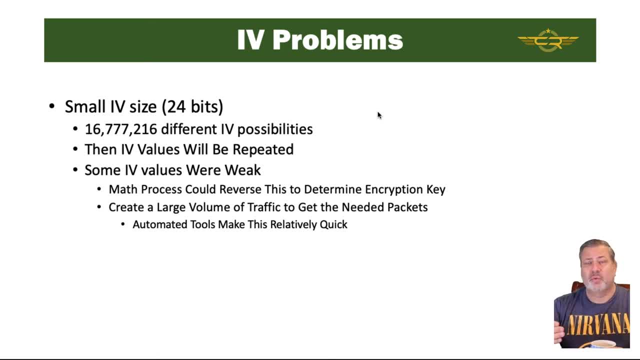 And we can use automated tools to make this relatively quick. So we can make this a lot faster using some automated tools to do this, And we'll see that with something like disassociation attacks and replay attacks, things like that, that will drive traffic up across the network. 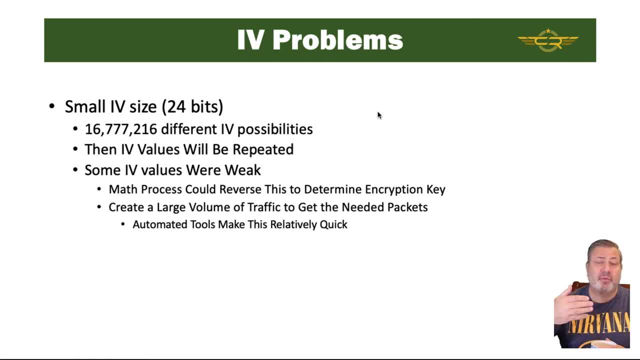 And that's what the bad guy, the attacker, is going to try to do. They're going to try to send a large volume of data across the network. Each time packets go across the network, they're going to have a different IV. 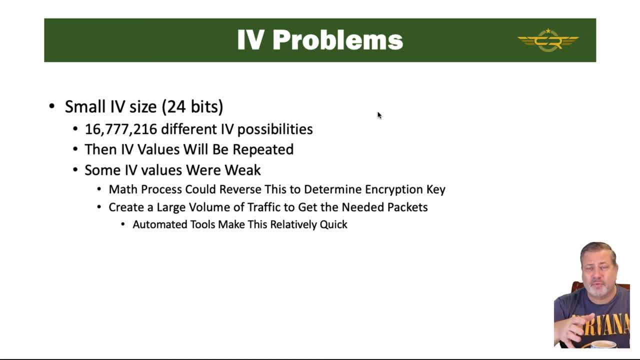 And really, as soon as we get to 15,000 or 20,000 different packets with different IVs, that's normally the range we need to be in to start getting repeated IV values: Right, Right, Right, Right Right. 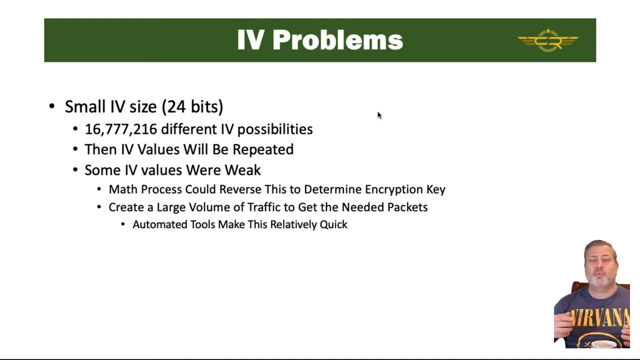 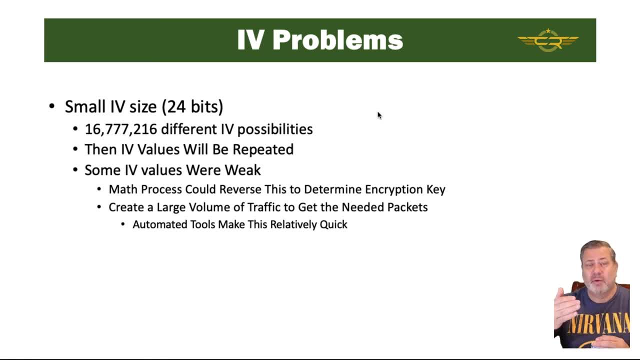 A lot of times this is done- I think, almost exclusively. this is done with tools that will help you do this, So you can push a lot of data across the network And then you can use that data to break the web key. That's why most new access points will not even allow you to use web, because it's so relatively insecure. 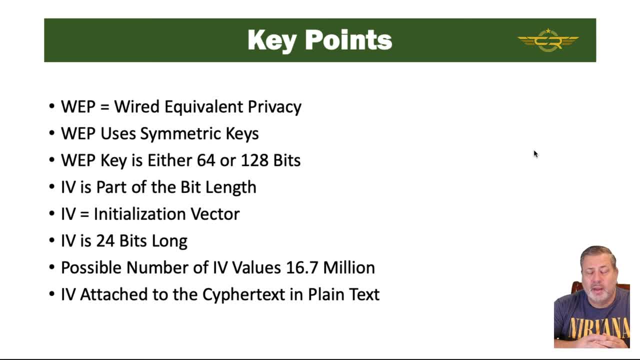 So when we're talking about this, when you're thinking about what you need to know for the exam, WEP is Wired- Equivalent Privacy. WEP uses symmetric keys. The WEP key is either going to be 64 or 128 bits long.